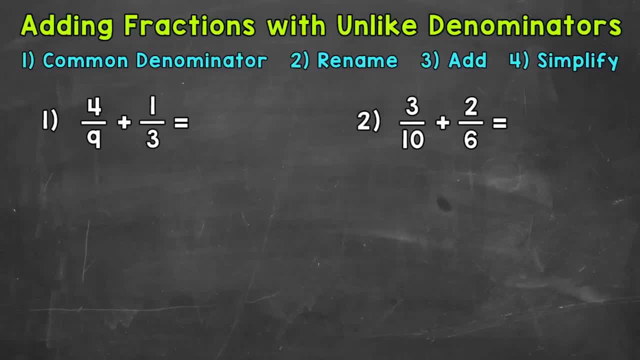 problem, but if not, you can always write out your lists of multiples in order to find it. Let's write out the multiples of nine and three, So I'll come to the bottom of the screen where I have some extra room to write out these lists. We'll start with nine, So nine. The first multiples of nine are nine. 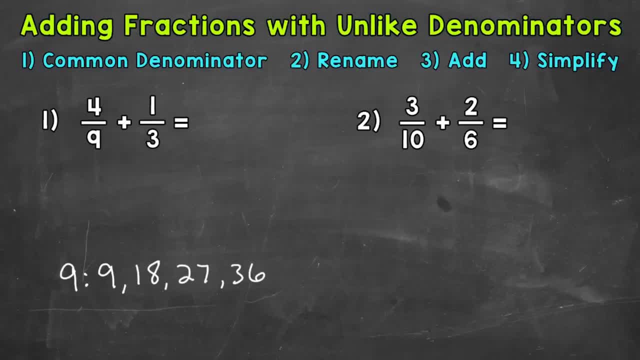 twenty-seven, thirty-six, So I'll write four multiples of nine there. I would suggest writing out four or five multiples of each. See if you have any common multiples, and if not, you can always extend your lists. So let's do three now and see if we have any common multiples. Three, six, nine. 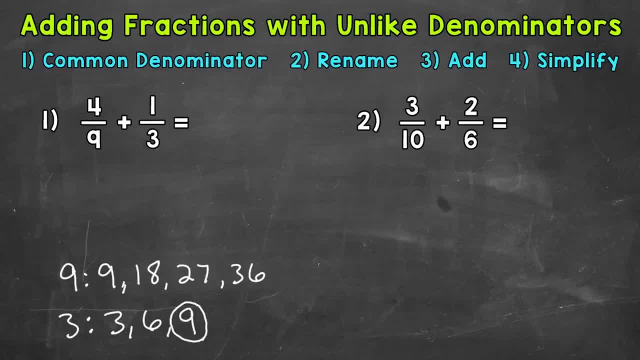 and it looks like we have a common multiple of nine And, more specifically, that's going to be the least common multiple. We always want to find the least common multiple. Smaller numbers in value are generally easier to work with and this will help cut down on simplifying in the end. So nine is going to be our common denominator. Let's come back up. 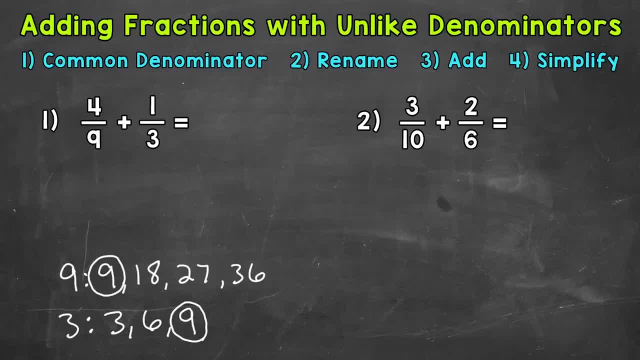 to the original problem and rename these fractions with our common denominator of nine. So underneath I'm going to write our common denominator of nine and now we can rename. So we'll start with four 9ths. Well, four 9ths already has a denominator of nine, so we don't need to rename. So we can just. 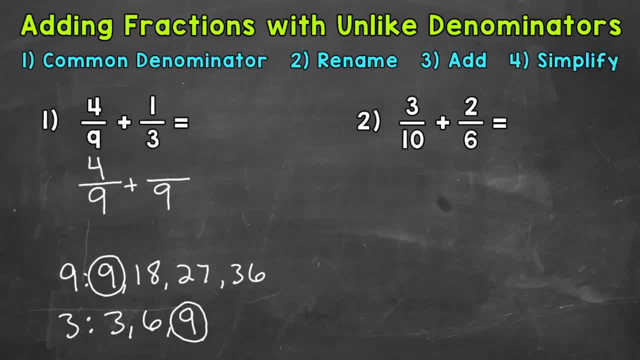 bring the four down As far as 1. 3rd, we need to think three times. what equals nine? How do we get three to equal nine? Well, we know three times three equals nine. Let's try this. We don't know that quite. yet. So we need to thinky thing as far as one-third. we need to think three times what equals nine? How do we get three to equal nine? Well, we know, three times three equals nine, and that's going to give us, instead of that, This is going to increasingly launch an instruction system. call of multiple numbers. 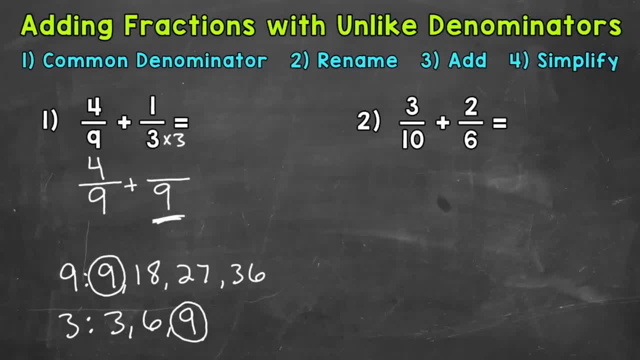 What again We're going to think of? the 9-7 is given, So what? I'm going to end up with dime a equals 9.. Now, in order to rename, we want to have an equivalent fraction. We want to keep this. 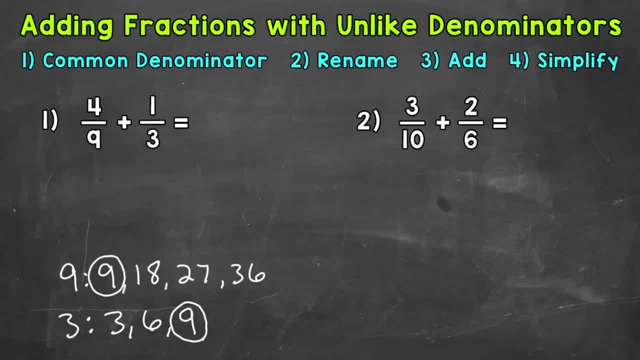 And more specifically that's going to be the least common multiple. We always want to find the least common multiple. Smaller numbers in value are generally easier to work with and this will help cut down on simplifying in the end. So nine is going to be our common denominator. Let's come back up to the original problem and rename these fractions with our common denominator of nine. So underneath I'm going to write our common denominator of nine and now we can rename. So we'll start with four ninths. Well four ninths already has a denominator of nine. So we don't need to rename. So we can just bring the four down. As far as 1 third, we need to think three times what equals nine. How do we get 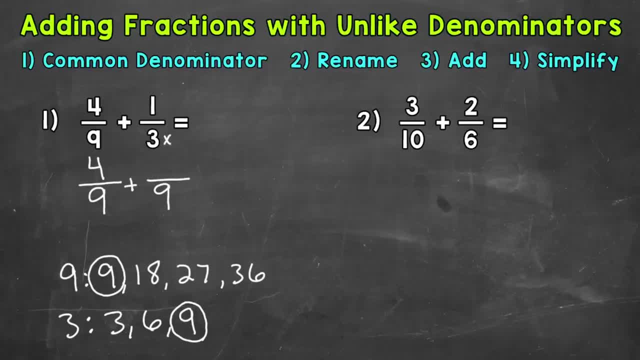 three to equal nine? Well we know three times three equals nine. Now this is not something that you can do in everyday practice. This is a very common denominator and when we're going to write a common denominator 9. Now in order to rename we want to have an equivalent fraction. We want to keep this equivalent. We do not want to change the value of the problem at all. So whatever we do to the denominator we have to do to the numerator. So 1 times 3 is 3. 3 ninths is equivalent to 1 third 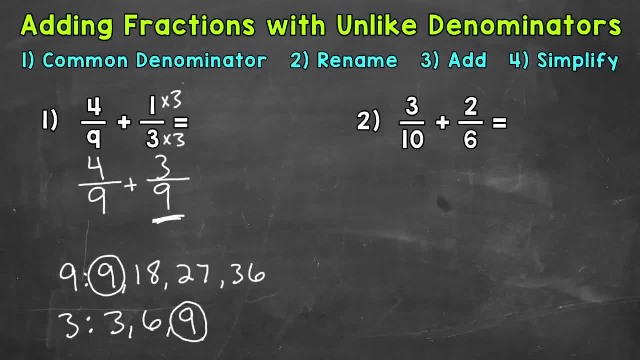 but we have that common denominator of 9 now. Now that both fractions have a common denominator we can add. So when we add fractions we add the numerators. The top numbers 4 plus 3 is 7 and then we keep the denominator the same. So 9. 7 ninths is our final answer. 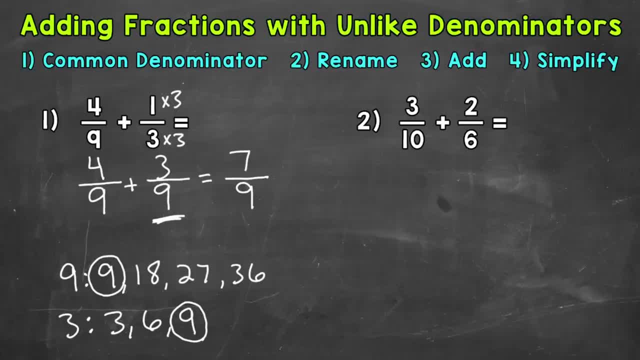 Now it's common practice to simplify fractional answers. 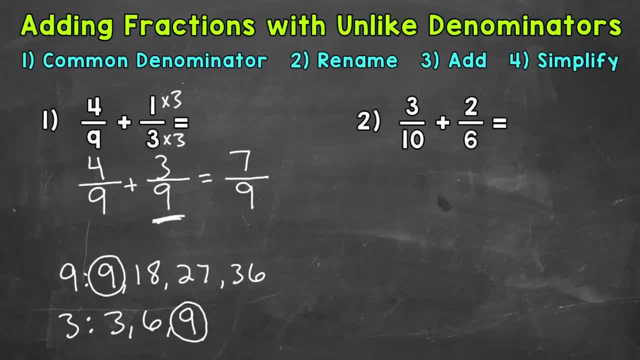 So we look to see if we can break this fraction down at all. Are there any common factors between 7 and 9 besides 1? Can we simplify? No. The only common factor between 7 and 9 is 1. So this is in simplest form and we are done. 7 ninths is our final answer. Let's try another one and move on 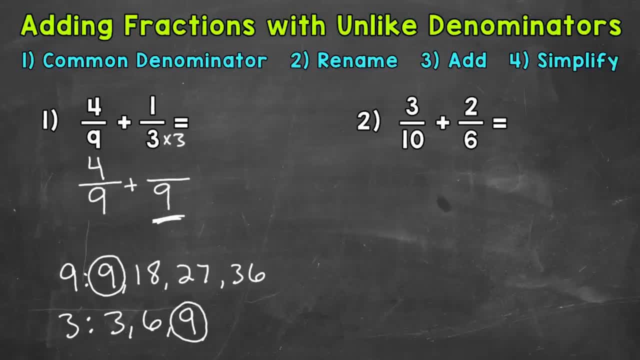 equivalent. We do not want to change the value of the problem at all. So whatever we do to the denominator, we have to do to the numerator. So 1 times 3 is 3.. 3 ninths is equivalent to 1 third. 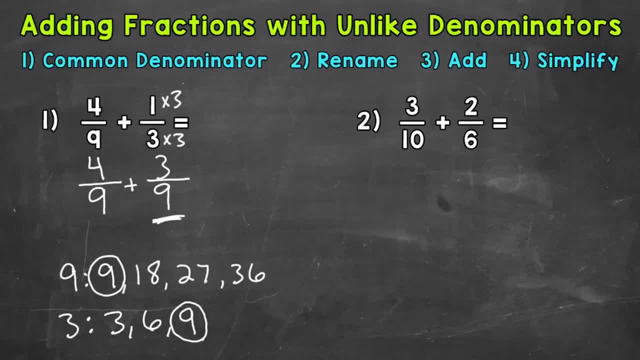 but we have that common denominator of 9 now, Now that both fractions have a common denominator, we can add. So when we add fractions, we add the numerators, The top numbers, 4 plus 3 is 7 and then we keep the denominator the same, So 9.. 7 ninths is our final answer. 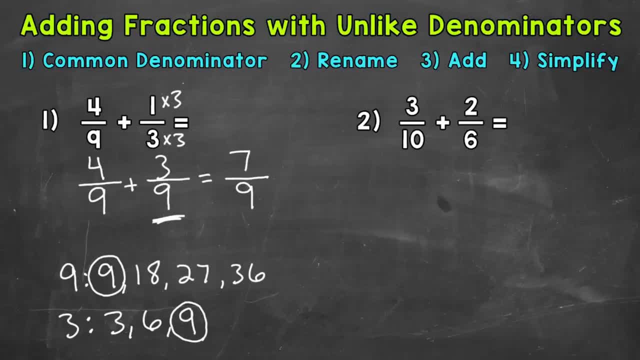 Now, it's common practice to simplify fractional answers, So we look to see if we can break this fraction down at all. Are there any common factors between 7 and 9 besides 1? Can we simplify? No, The only common factor between 7 and 9 is 1.. So this is in. 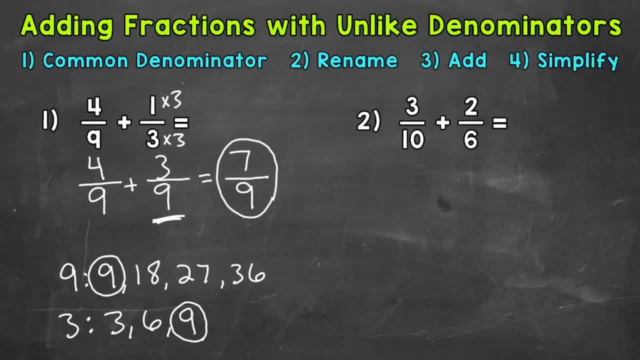 simplest form and we are done. 7 ninths is our final answer. Let's try another one and move on to number 2, where we have 3 tenths plus 2 sixths. So the first thing that we want to do is to: 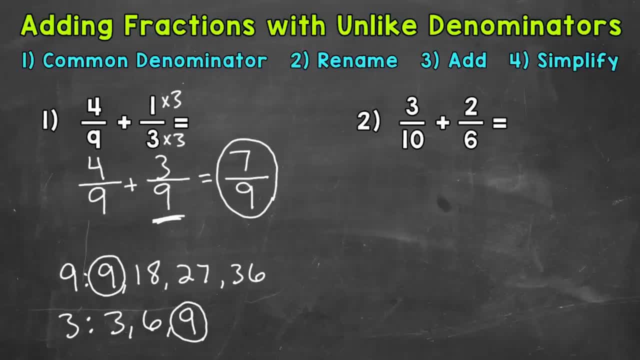 find a common denominator. So let's write out the multiples of 10 and 6.. We'll start with 10.. So 10, 20,, 30,, 40.. So we'll write out 4 multiples for each. Let's do 6 now. 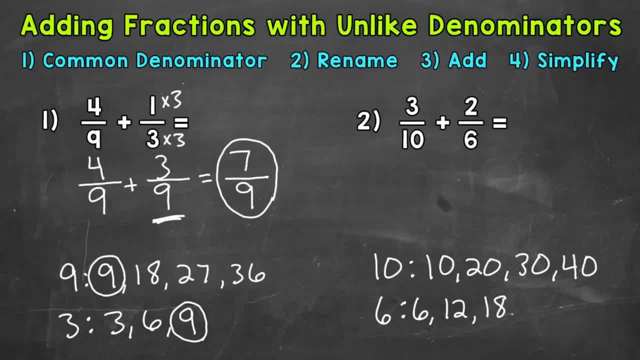 6, 12,, 18,, 24.. So 4 for each and we don't have a common multiple. That's okay, We can extend our lists. Now the multiples of 10 were already at 40 and the multiples of 6 were only at 24.. So let's extend that list. So after 24 would be 30, and now we have. 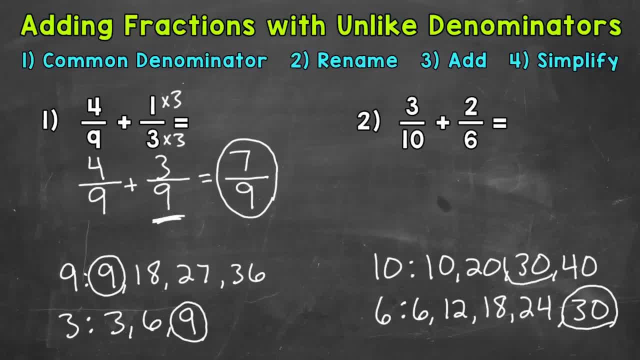 a common multiple and specifically the least common multiple. So 30 is going to be our common denominator. Let's rename our fractions with that denominator of 30.. Let's start with 3 tenths. So we need to think: how do we get 10 to equal 30? 10 times what? 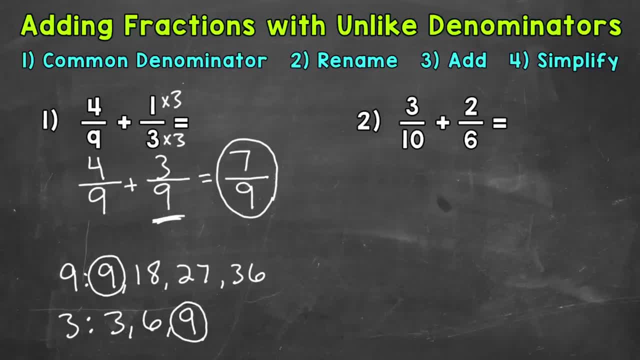 to number 2 where we have 3 tenths plus 2 sixths. So the first thing that we want to do is to find a common denominator. So let's write out the multiples of 10 and 6. We'll start with 10. So 10, 20, 30, 40. So we'll write out 4 multiples for each. Let's do 6 now. 6, 12, 18, 24. So 4 for each and we don't have a common multiple. 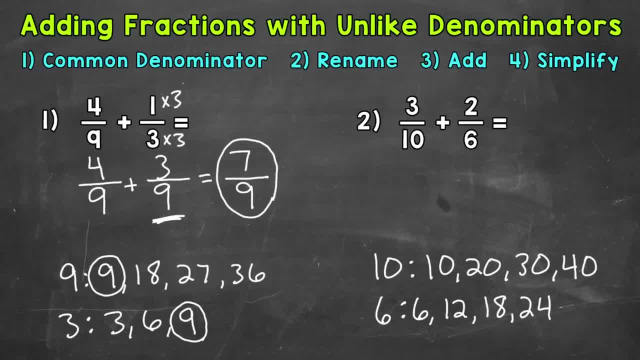 That's okay. We can extend our lists. Now the multiples of 10 were already at 40 and the multiples of 6 were only at 24. So let's extend that list. So after 24 would be 30 and now we have a common multiple and specifically the least common multiple. So 30 is going to be our common denominator. Let's rename our fractions with that denominator. 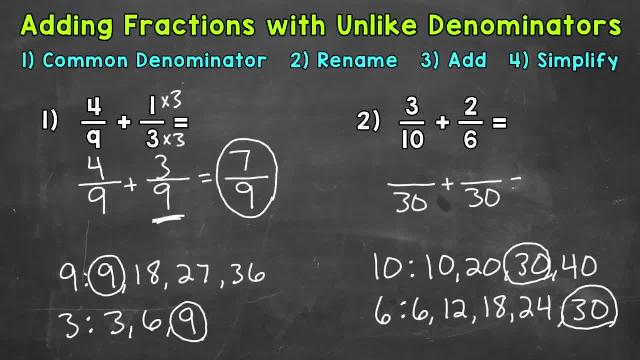 of 30. Let's start with 3 tenths. So we need to think how do we get 10 to equal 30? 10 times what equals 30? Well 10 times 3 equals 30. We know 10 times 3 equals 30. In order to keep this equivalent whatever we do to the denominator we have to do to the numerator. So multiply the numerator by 3 as well. 3 times 3. 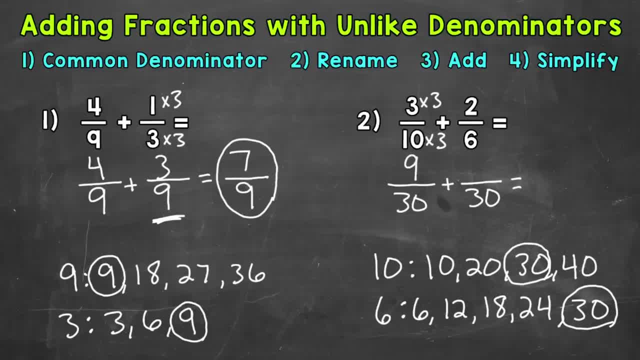 is 9. So 9 thirtieths is equivalent to 3 tenths. But we have that common denominator of 30 now. Now we do 2 sixths. So we think how do we get 6 to equal 30? 6 times what is 30? Well 6 times 5 is 30. 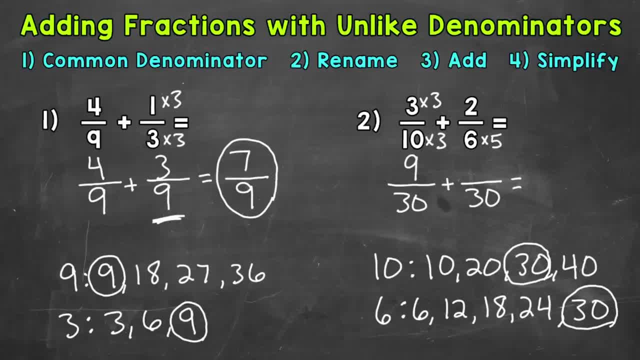 Whatever we do to the denominator we do to the numerator. So 2 times 5 gives us 10. 10 thirtieths is equivalent to 2 sixths. 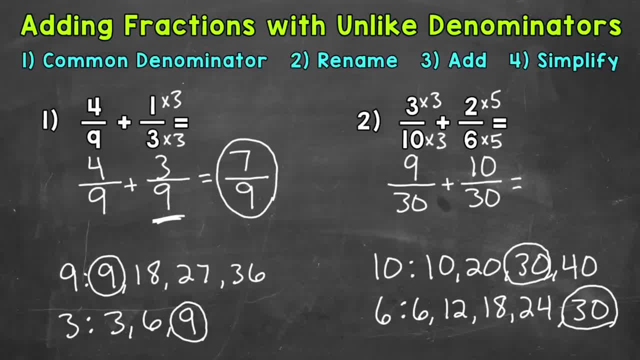 Now that we found the common denominator we renamed we can add. So add the numerators. 9 plus 10 is 19. 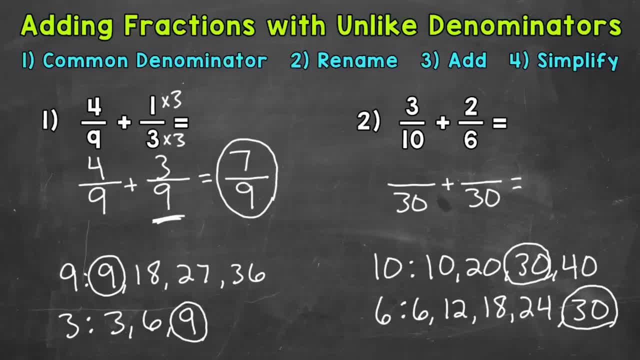 equals 30?? Well, 10 times 3 equals 30. We know 10 times 3 equals 30. In order to keep this equivalent, whatever we do to the denominator, we have to do to the numerator. So, multiply the numerator by 3. 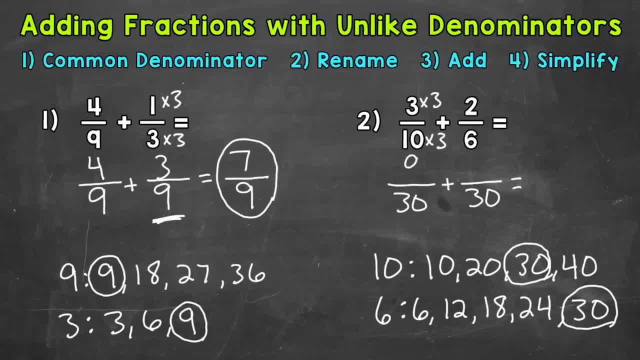 as well. 3 times 3. is 9.. So 9 thirtieths is equivalent to 3 tenths, But we have that common denominator of 30 now. Now we do 2 sixths. So we think: how do we get 6 to equal 30?? 6 times what is 30?? Well, 6 times 5 is 30. 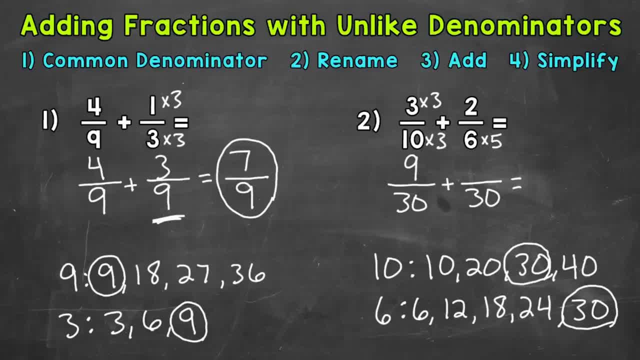 Whatever we do to the denominator, we do to the numerator. So 2 times 5 gives us 10.. 10 thirtieths is equivalent to 2 sixths. Now that we found the common denominator, we renamed, we can add. So add the numerators: 9 plus 10 is 19.. 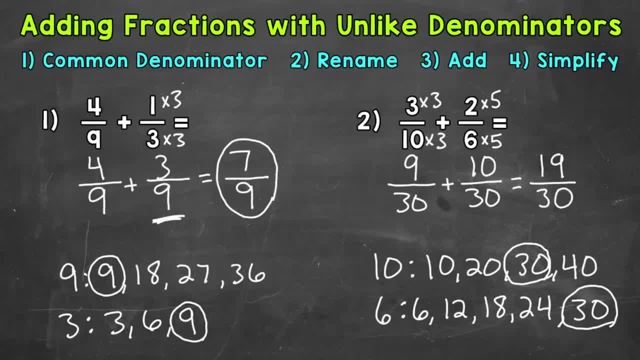 Keep the denominator of 30. And our final answer is 19 thirtieths. We can check to see if we can simplify, But 19 thirtieths is in simplest form. The only common factor between 19 and 30 is 1.. So we are done. 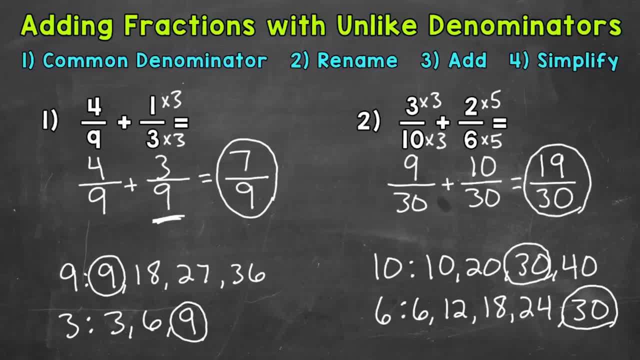 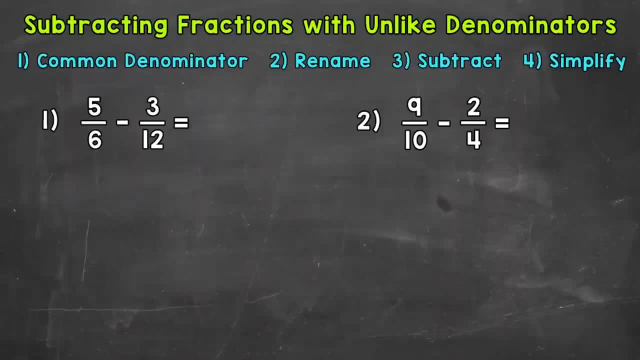 So there you have it. There's how you add fractions with unlike denominators. Let's move on to subtraction and try two of those examples as well. We'll start with number 1, where we have 5 sixths minus 3 twelfths, And just like: 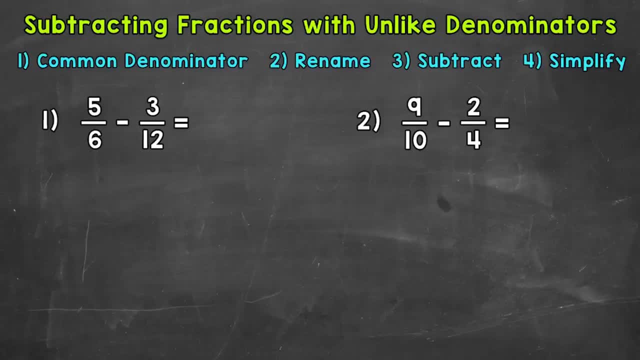 adding fractions with unlike denominators. when we subtract, we need a common denominator. for number one, we have a 6 and a 12. So we don't have a common denominator to start with. So we can't subtract quite yet. The first thing that we need to do is find a common denominator, and we can do that by. 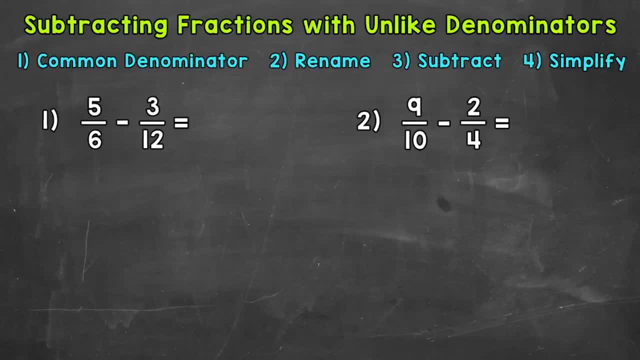 finding the least common multiple between our denominators. We want the least because smaller numbers in value are generally easier to work with and this will help cut down on simplifying in the end. once we get to our answer As far as why we need a common denominator, that's a topic. 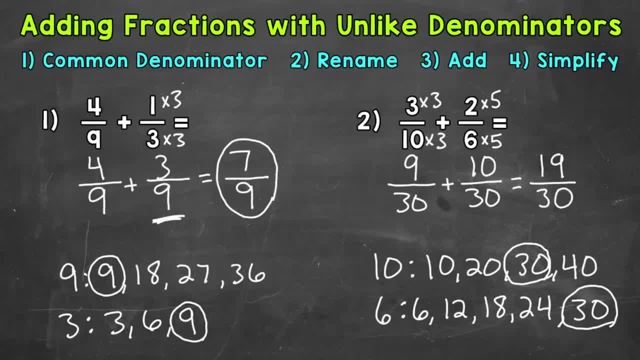 Keep the denominator of 30. And our final answer is 19 thirtieths. We can check to see if we can simplify. But 19 thirtieths is in simplest form. The only common factor between 19 and 30 is 1. So we are done. 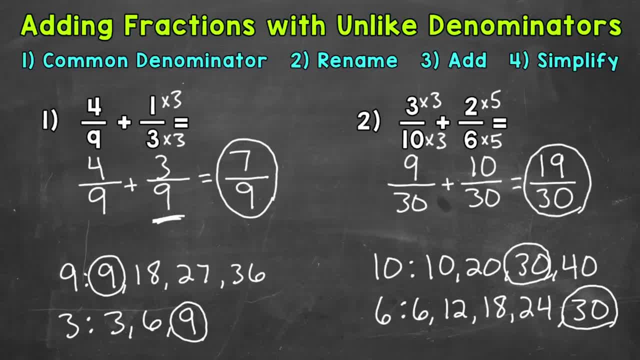 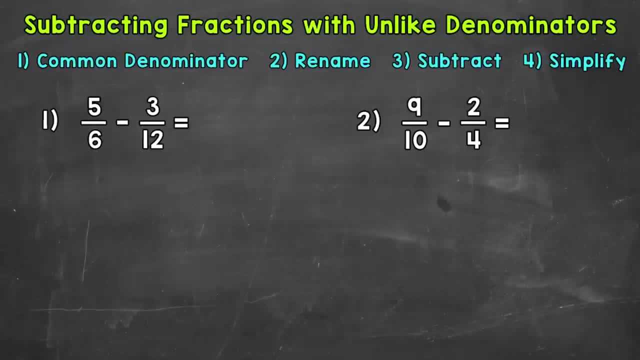 So there you have it. There's how you add fractions with unlike denominators. Let's move on to subtraction and try 2 of those examples as well. We'll start with number 1 where we have 5 sixths minus 3 twelfths. And just like adding fractions with unlike denominators when we subtract we need a common denominator. 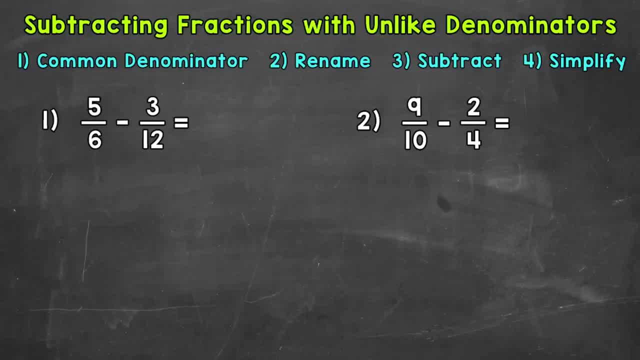 For number 1 we have a 6 and a 12. So we don't have a common denominator to start with. So we can't subtract quite yet. The first thing that we need to do is find a common denominator. And we can do that by finding the least common multiple between our denominators. We want the least because smaller numbers in value are generally easier to work with. And this will help cut down on simplifying in the end once we get to our answer. 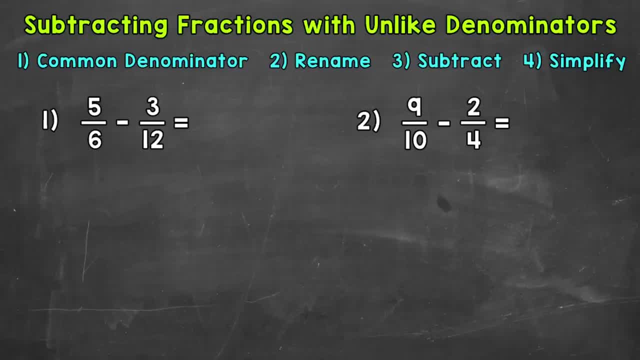 As far as why we need a common denominator, that's a topic for another video. I'll drop that link down in the description. Now as you're looking at a subtraction problem involving fractions with unlike denominators, you may recognize the least common multiple between denominators right away. 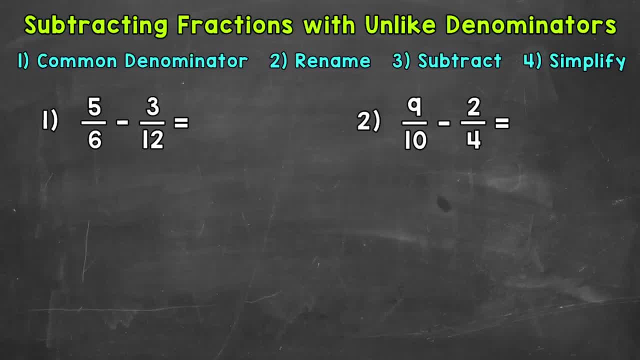 But if not, you can always write out your lists of multiples in order to find it. 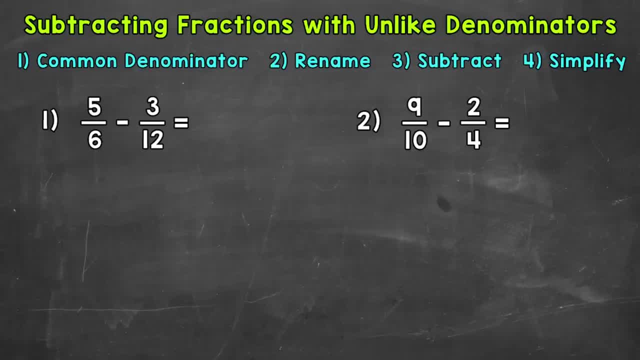 So let's start by writing some multiples of both 6 and 12. And see if we can find that least common. We'll start with 6, so I'm going to come to the bottom of the screen where I have some extra room to write out these lists and we'll start with 6. So I would suggest writing out 4 or 5 multiples for each denominator and see if you can find that least common multiple. If not, you can always extend the lists until you find that least common multiple. So if 4 or 5 multiples don't work and you don't see any common multiples, Extend those lists. So the first four multiples of 6 are 6, 12, 18, 24. 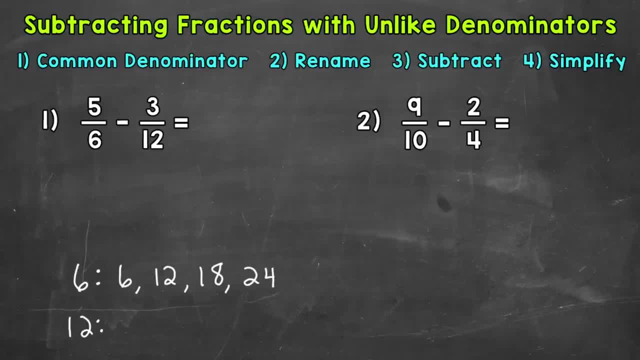 Now we'll do 12. The first multiple of 12 is 12. 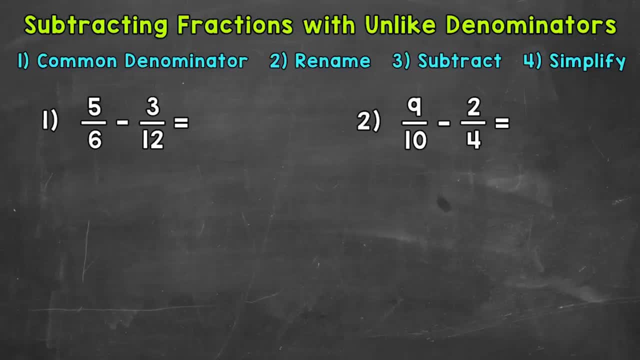 for another video. I'll drop that link down in the description Now, as you're looking at a subtraction problem involving fractions with unlike denominators. you may recognize the least common multiple between denominators right away, but if not, you can always write out your lists. 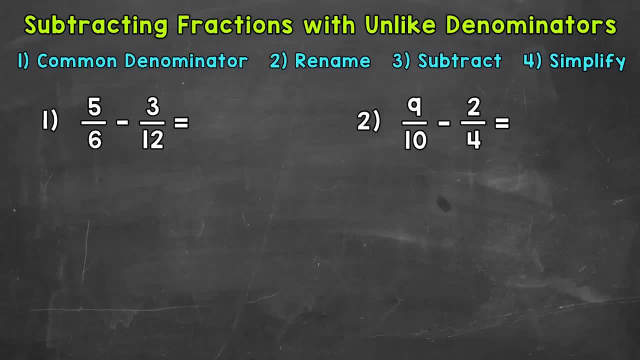 of multiples in order to find it. So let's start by writing some multiples of both 6 and 12 and see if we can find that least common multiple. We'll start with 6, so I'm going to come to the bottom of the screen where I have some extra room to write out these lists, and we'll 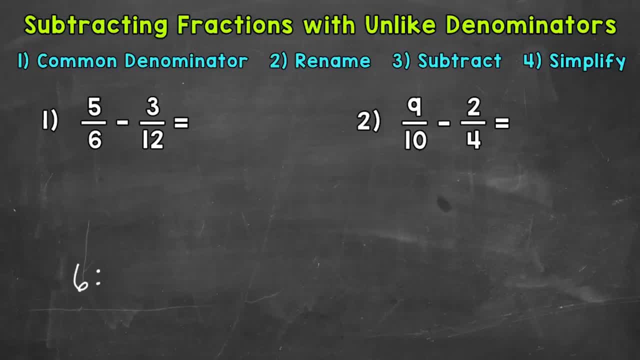 start with 6.. So I would suggest writing out 4 or 5 multiples for each denominator and see if you can find that least common multiple. If not, you can always extend the lists until you find that least common multiple. So if 4 or 5 multiples don't work and you don't see any common multiples, 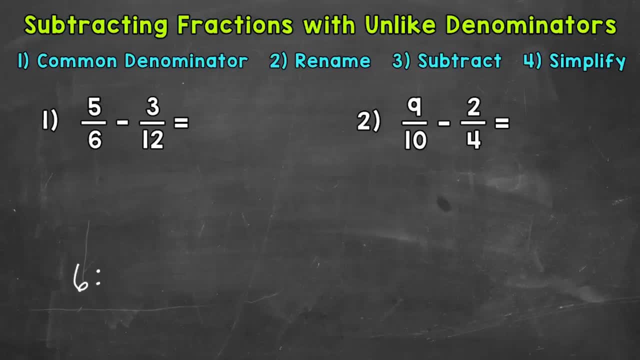 extend those lists. So the first 4 multiples of 6, are 6,, 12,, 18,, 24.. Now we'll do 12.. So the first multiple of 12 is 12.. Now, no need to go on if you. 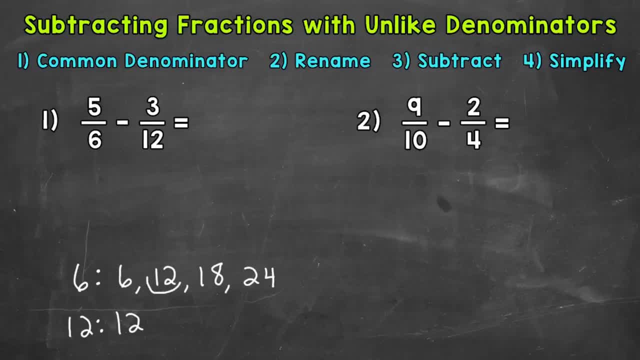 find that least common multiple because if you look, we have a least common multiple of 12.. So we are ready to move to the next step, which is rename. So 12 is going to be our common denominator. I'm going to come back up to the original problem underneath and start to write the renamed. 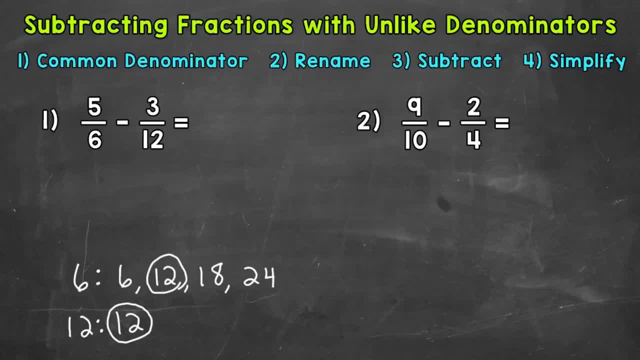 fractions with that common denominator of 12.. So underneath I'll start these fractions with that common denominator of 12 and now we're going to rename. We'll start with 5 sixths, so we're going to rename that fraction with an equivalent fraction with the denominator of 12.. So we need to think. 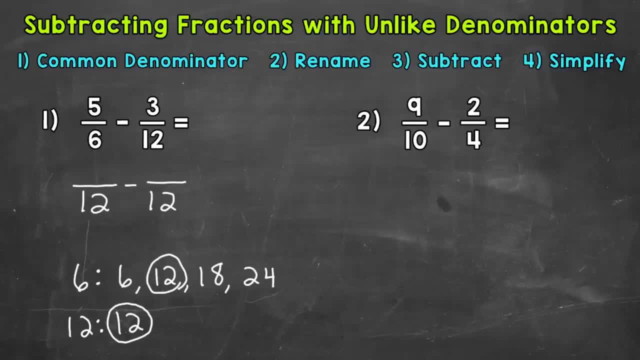 How do we get the denominator of 12?? Well, let's start with the denominator of 12, and we'll start of 6 to equal the denominator of 12.. 6 times what equals 12?? Well, we know that: 6 times 2. 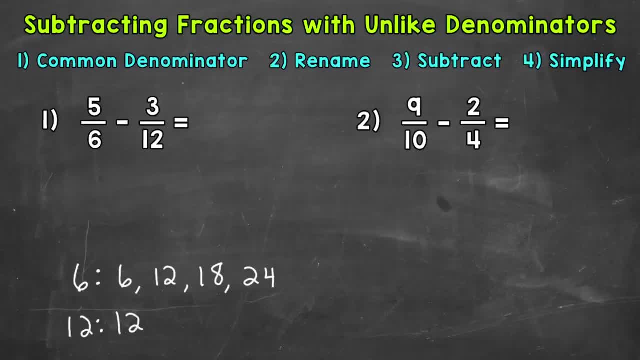 No need to go on if you find that least common multiple. Because if you look, we have a least common multiple of 12. 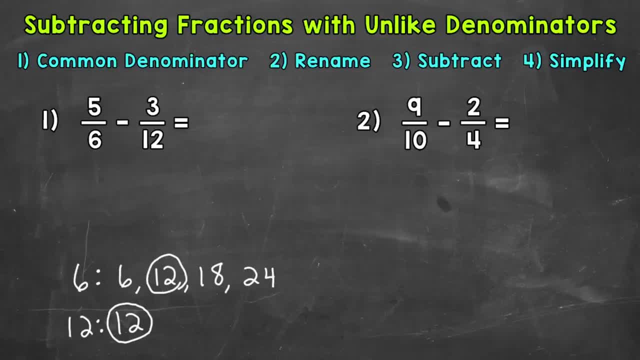 So we are ready to move to the next step. is rename. So 12 is going to be our common denominator. I'm going to come back up to the original problem underneath and start to write the renamed fractions with that common denominator of 12. So underneath I'll start these fractions with that common denominator of 12 and now we're going to rename. We'll start with 5 sixths. So we're going to rename that fraction with an equivalent fraction with the denominator of 12. So we need to think how do we get the denominator of 6 to equal the denominator of 12? 6 times what equals 12? Well we know that 6 times 2 equals 12. 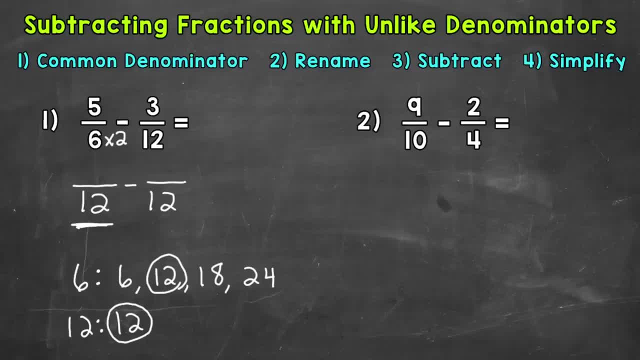 So whatever we do to the denominator, the bottom number, we have to do to the numerator, the top number, in order to keep this fraction equivalent. We don't want to change the value of the denominator. We want to keep the denominator equivalent. So we're going to of the problem at all. So we need to do 5 times 2 to get the renamed numerator. 5 times 2 is 10. So 10 twelfths is equivalent to 5 sixths. So we renamed with that denominator of 12. 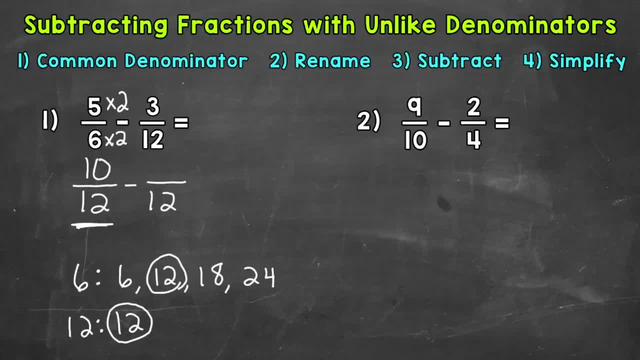 Now we need to do 3 twelfths. Well 3 twelfths already has a denominator of 12. So we don't need to rename. We can just bring the 3 down. Once we rename, we can subtract. When we subtract fractions, we subtract the numerators. So 10 minus 3 is 7. And then we keep the denominator of 12 the same. So 7 twelfths is our answer. Now always look to 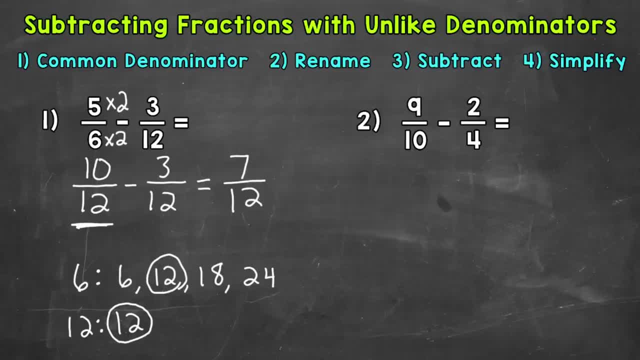 simplify. So can we simplify 7 twelfths? Well 7 twelfths is in simplest form. The only common factor between 7 and 12 is 1. So we can keep the denominator of 12 the same. So 7 twelfths is our answer. Now always look to simplify. So can we simplify 7 twelfths? Well 7 twelfths is in simplest form. The only common factor between 7 and 12 is 1. So we can't break this down any further as far as simplifying goes. So our final simplified answer, 7 twelfths. Let's try another one and move 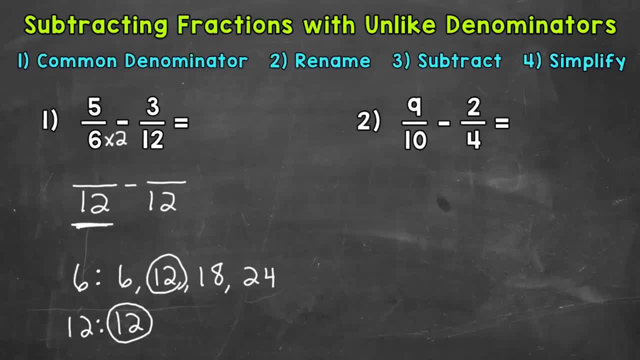 equals 12.. So whatever we do to the denominator- the bottom number, we have to do to the numerator- the top number, in order to keep this fraction equivalent. We don't want to change the value of the problem at all. So we need to do 5 times 2 to get the renamed numerator. 5 times 2. 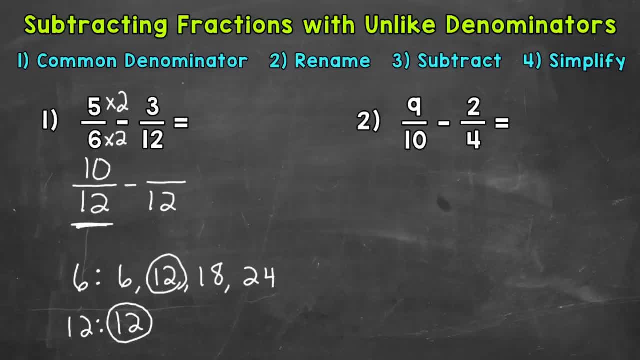 is 10.. So 10 twelfths is equivalent to 5 sixths. So we renamed with that denominator of 12.. Now we need to do 3 twelfths. Well, 3 twelfths already has a denominator of 12,. 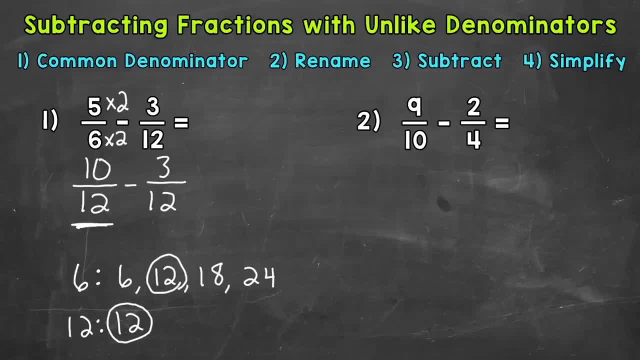 so we don't need to rename, We can just bring the 3 down. Once we rename, we can Subtract. When we subtract fractions, we subtract the numerators. So 10 minus 3 is 7.. And then we keep the denominator of 12 the same, So 7 twelfths is our answer. 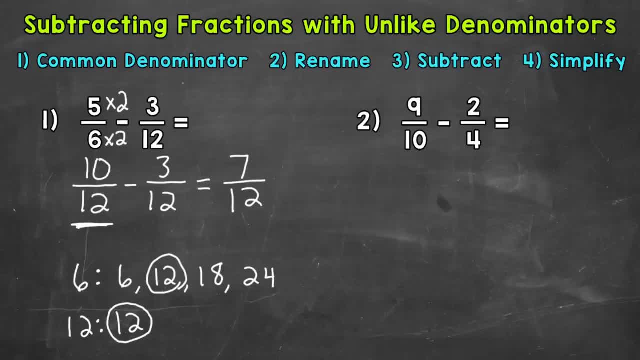 Now always look to simplify. So can we simplify 7 twelfths? Well, 7 twelfths is in simplest form. The only common factor between 7 and 12 is 1.. So we can. We can't break this down any further as far as simplifying goes. So our final simplified answer: 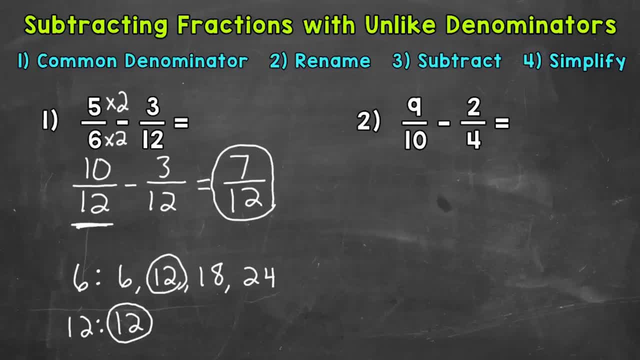 7 twelfths. Let's try another one and move on to number 2, where we have 9 tenths minus 2 fourths. So the first thing that we need to do find a common denominator. So we need that least. 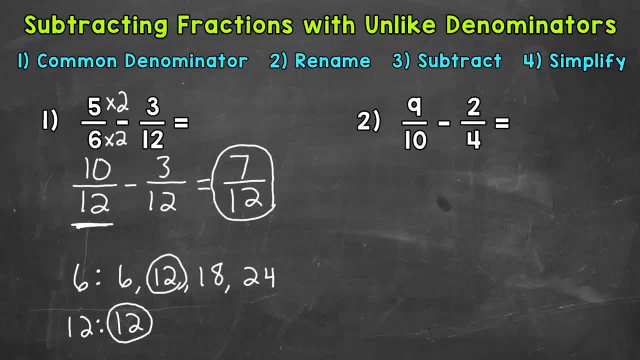 common multiple between 10 and 4, and that's going to be our common denominator. Let's go down to the bottom and write out The multiples. So we'll start with 10, and we'll write out 4 multiples to start with. 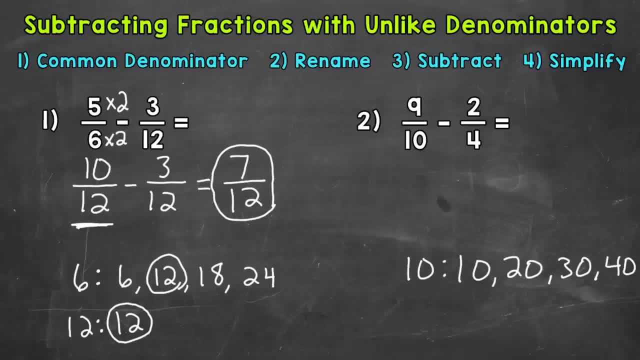 So 10, 20,, 30, 40. Now let's write out 4 multiples of 4 and see if we have a least common multiple. So 4, 8,, 12, 16.. So writing out 4 multiples for each, we don't have a match, So we need to. 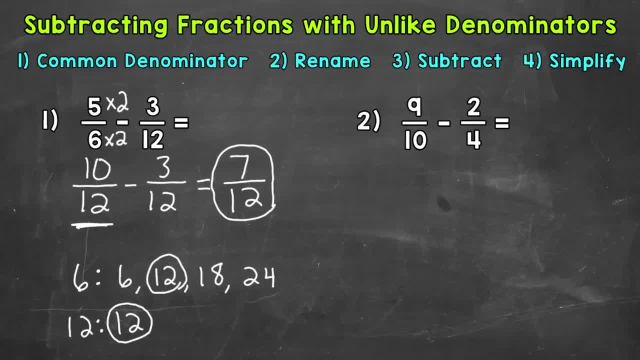 on to number 2, where we have 9 tenths minus 2 fourths. So the first thing that we need to do, 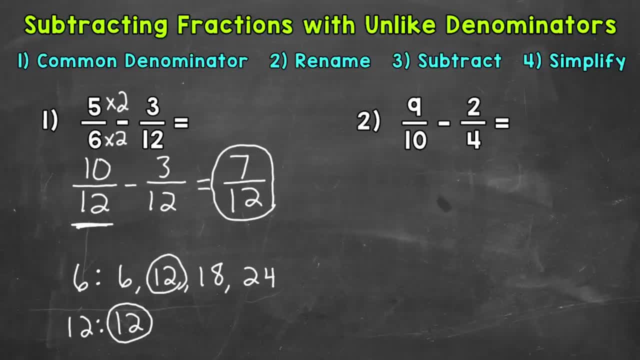 find a common denominator. So we need that least common multiple between 10 and 4, and that's going to be our common denominator. Let's go down to the bottom and write out, some multiples. So we'll start with 10, and we'll write out 4 multiples to start with. So 10, 20, 30, 40. Now let's write out 4 multiples of 4 and see if we have a least common multiple. So 4, 8, 12, 16. So writing out 4 multiples for each, we don't have a match. So we need to extend our lists. Now the multiples of 10, we are already at 40. And the multiples of 4, we're only at 16. So let's extend that one. And the next multiple of 4 is 20. And that's going to give us a common multiple, and specifically the least common multiple. So we're going to use 20 for our common denominator. Let's go back up to the original problem underneath and rename, with that common denominator of 20. We'll start with 9 tenths. So how do we get that denominator of 10 to equal 20? Well, 10 times 2 is 20. And whatever we do to the denominator, we have to do to the numerator in order to keep this equivalent. So 9 times 2 gives us 18 for our renamed numerator. 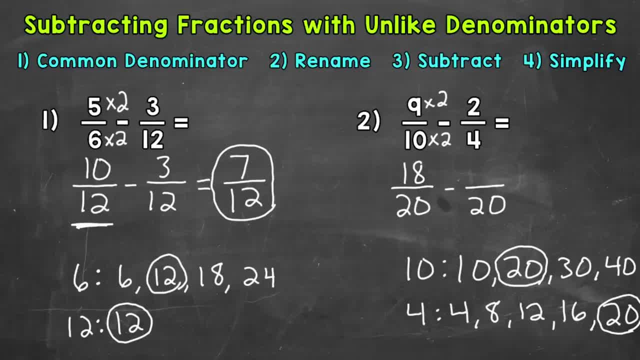 So 9 times 2 is equivalent to 9 tenths. We just have that common denominator of 20 now. Now we need to do 2 fourths. So how do we get 4 to equal 20? Well, we know 4 times 5 equals 20. So 4 times 5 equals 20. So we need to do the same thing to the numerator in order to get that renamed equivalent fraction with the denominator of 20. So same thing to the numerator. 2 times 5 gives us 10. 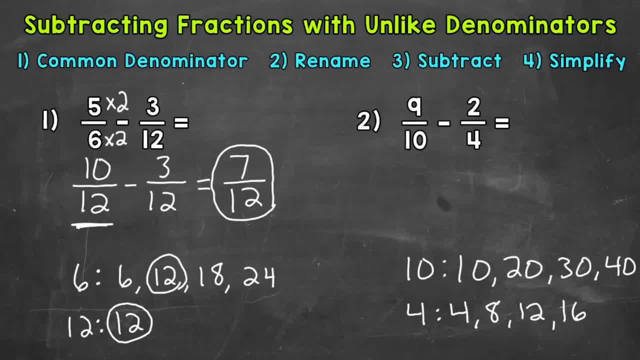 extend our lists Now: the multiples of 10, we are already at 40.. And the multiples of 4, we're only at 16.. So let's extend that one, And the next multiple of 4 is 20.. And that's going to give us 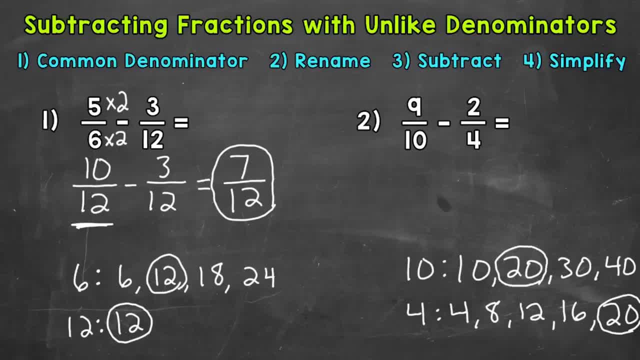 a common multiple and specifically the least common multiple. So we're going to use 20 for our common denominator. Let's go back up to the original problem underneath and rename with the common denominator of 20.. We'll start with 9 tenths. So how do we get that denominator of 10? 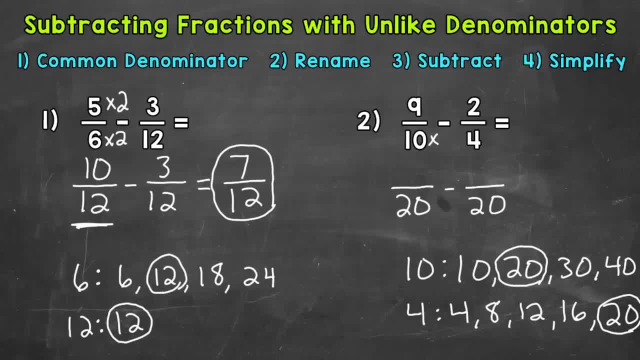 to equal 20?? Well, 10 times 2 is 20.. And whatever we do to the denominator, we have to do to the numerator in order to keep this equivalent. So 9 times 2 gives us 18 for our renamed numerator. 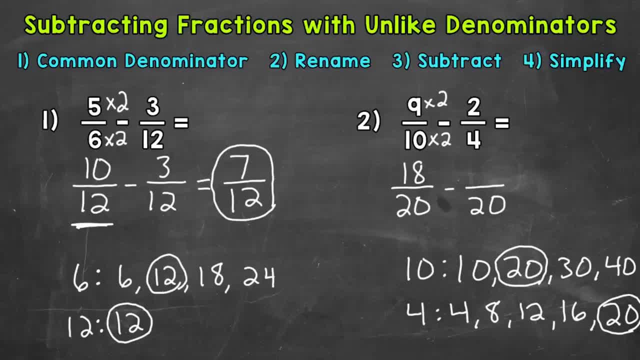 So 18 twentieths is equivalent To 9 tenths. We just have that common denominator of 20 now. Now we need to do 2 fourths. So how do we get 4 to equal 20?? Well, we know, 4 times 5 equals 20.. So 4 times 5 equals 20.. So we need to. 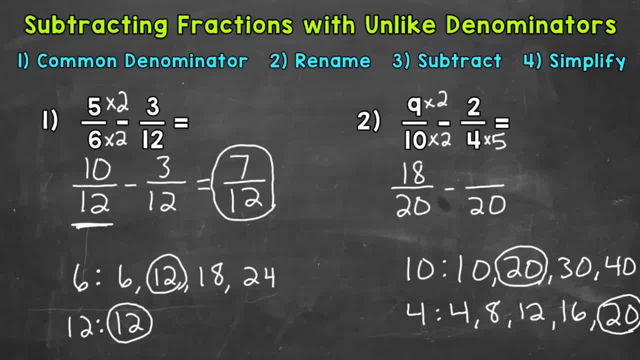 do the same thing to the numerator in order to get that renamed equivalent fraction with the denominator of 20.. So same thing to the numerator: 2 times 5 gives us 10.. Now we're ready to subtract. So subtract the numerators, the top numbers: 18 minus 10 is 8.. 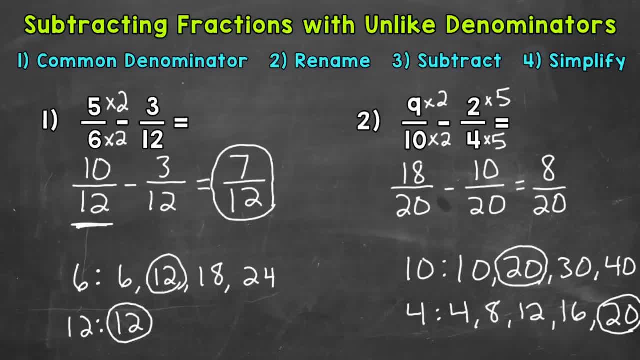 Keep the denominator of 20.. And our final answer is 8 twentieths. Now, 8 twentieths can be simplified. There are multiple paths that we can take in order to get this into simplest form, But if we use the greatest common factor between 8 and 20, we can simplify it. 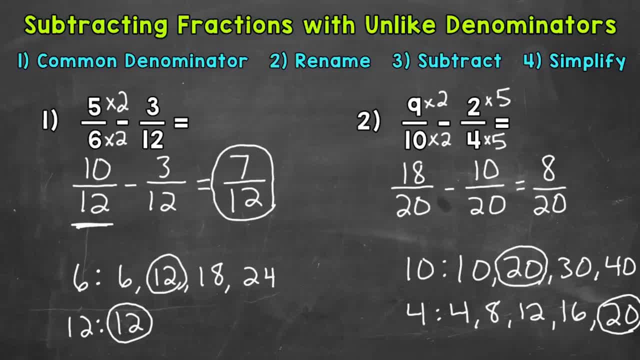 We have 3,, 4,, 8,, 5,, 2, and d cult. We can write 4 as winning numbers in order to get your final answer. So now we have 7 coins and after doing this, our answer should always be 4, but I'm going to give you four HOW to simplest answer numbers. 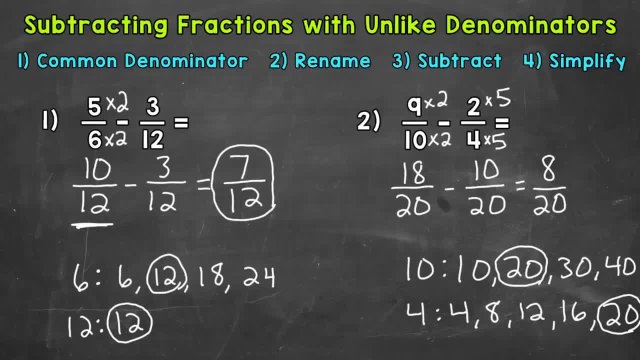 The great most common factor between 8 and 20 is 4.. So let's divide both of these to get our simplified answer number in order to get our simplified answer. So 8 divided by 4, and 20 divided by 4..